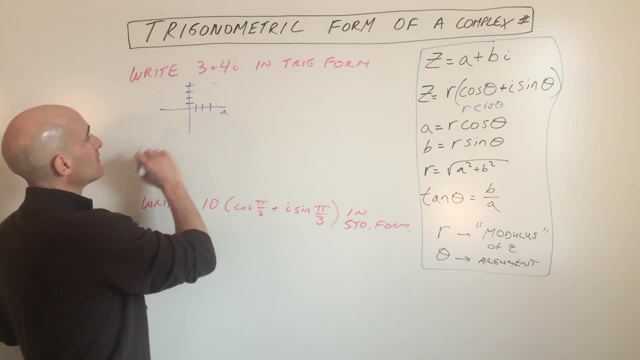 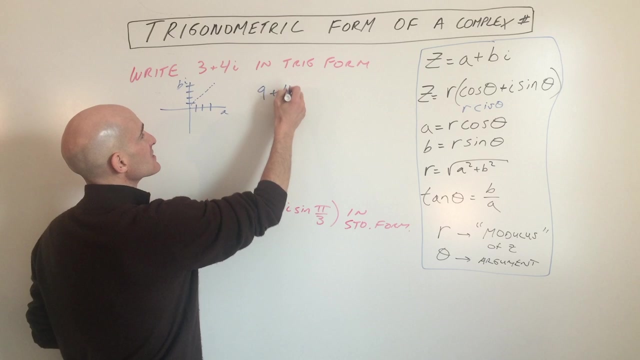 there's 3 plus 4i plotted in the complex plane, like the real and imaginary plane here, And what we're doing is we're finding this distance, okay from here, the origin to this point. And so what you can do is you can do the Pythagorean theorem or you can use this formula here: square root of a squared plus b squared, So this is going to be 9 plus 16.. Take the square root, That gives us 5.. Okay, now to find 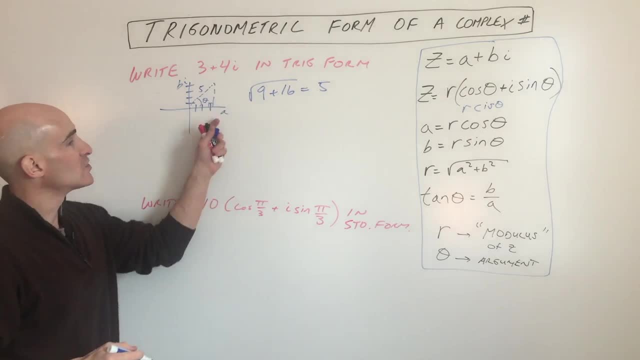 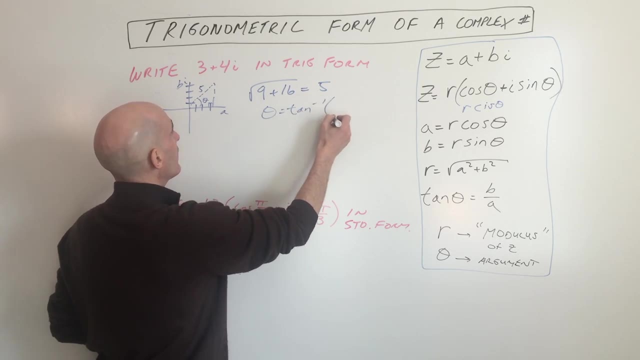 this angle, theta. okay, what we can do is we can use tangent inverse of b over a. So theta equals the tangent inverse of b, which is 4, over 3.. So let's do that in the calculator and see what that. 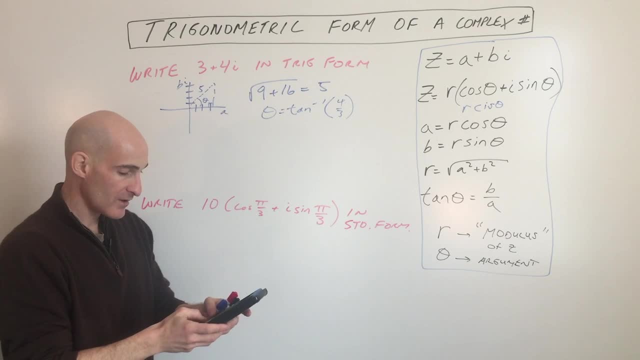 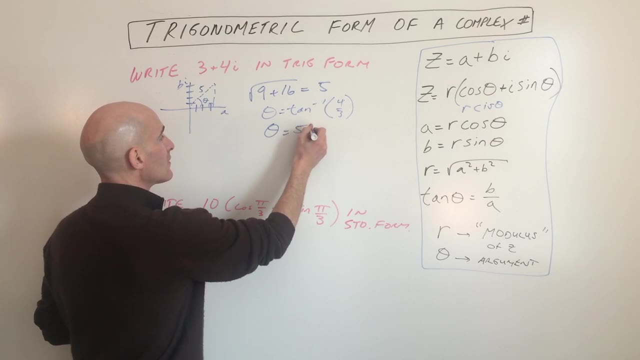 comes out to Tangent inverse of 4 divided by 3, which is 53.1.. Okay, so we've got 53.1 degrees. So if we're going to write this in trigonometric form, we've got 5. 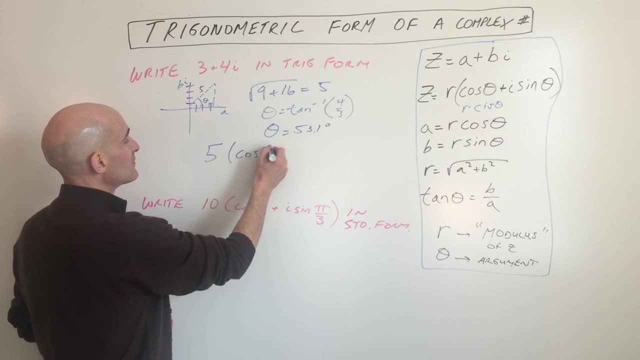 cosine 53.1 plus i sine 53.1.. And there's your trigonometric form. So we found this r value, okay, which is like the distance from the origin to the point in the complex plane there, And then we found the angle that it makes here with the positive x-axis. Okay, now we're going to go from. 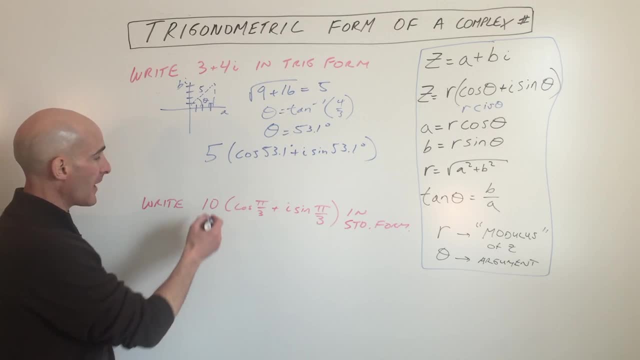 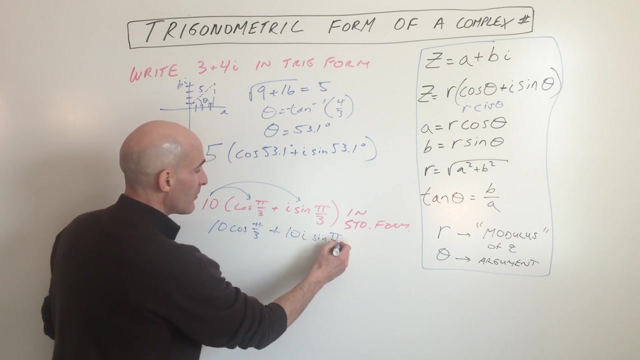 the trigonometric form to standard form. So how do we do that? What we're going to do is we're going to think about distributing this r value to the cosine and the sine. So that's going to give us 10 cosine pi over 3 plus 10 i sine pi over 3.. Pi over 3, cosine pi over 3 is a half times 10.. 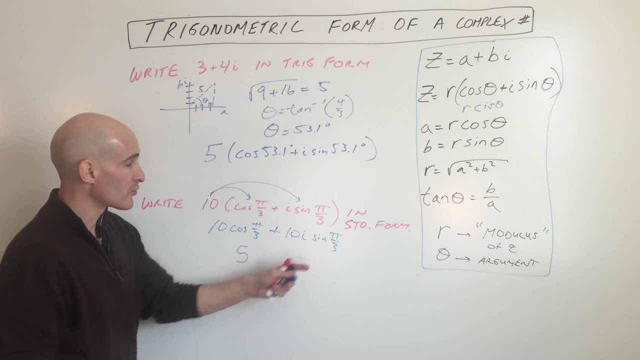 We'll give you 5.. Sine, pi over 3 is square root 3 over 2.. So that's going to give you, let's see so, 10 times square root 3 over 2. i But the 2 and the 10, you can see, reduce. 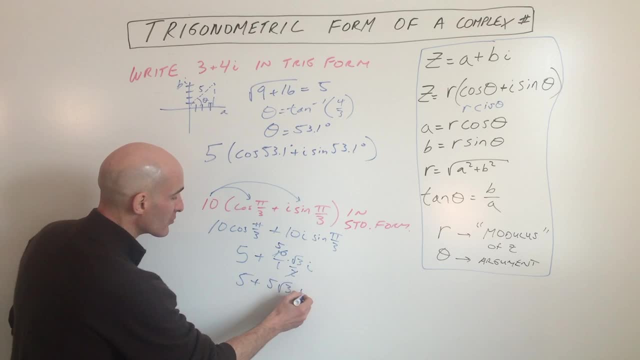 So that's going to give you 5 plus 5 square root of 3: i. So now we're back into the standard form.